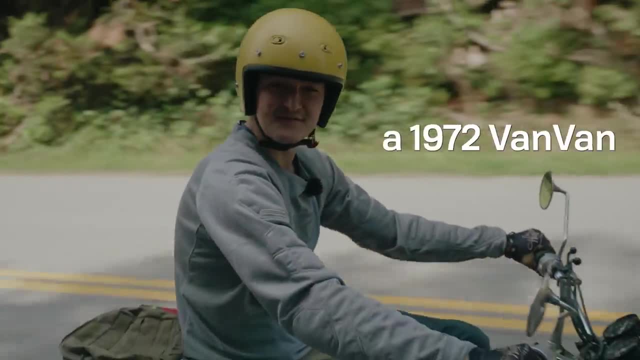 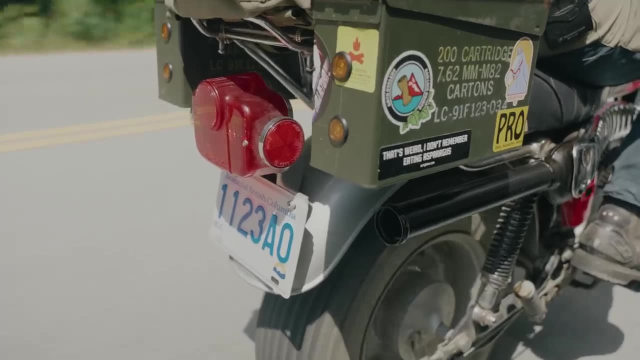 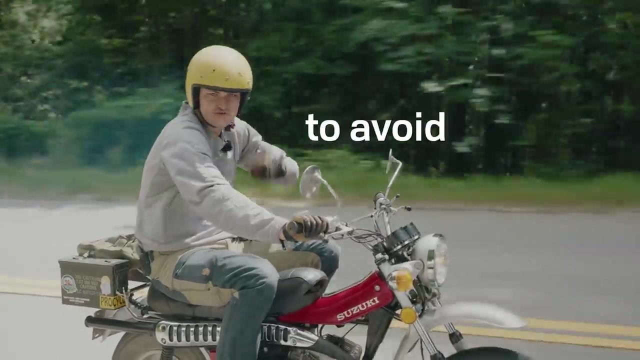 Good morning. I've come to you from the banana seat of a 1972 Van Band. at oh 7,000 o'clock, Old two-strokers would say. I'm on the bike riding with enough airflow to avoid oil fouling a spark plug. 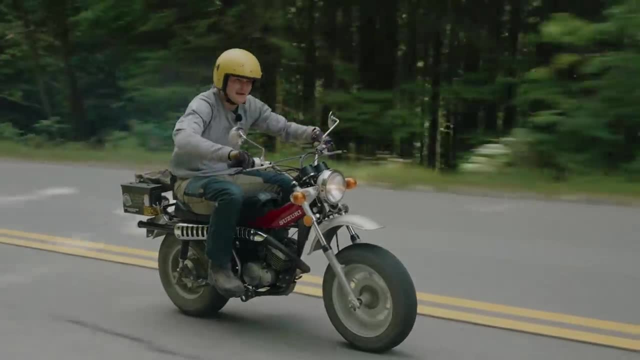 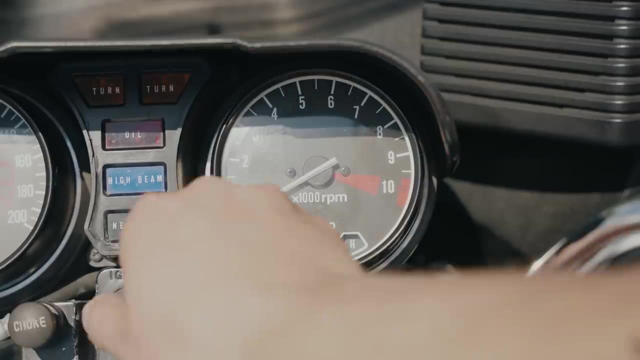 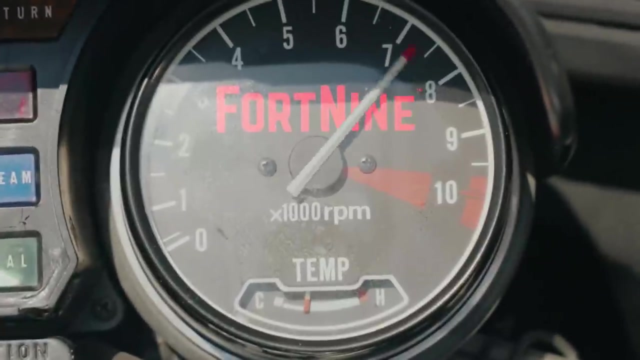 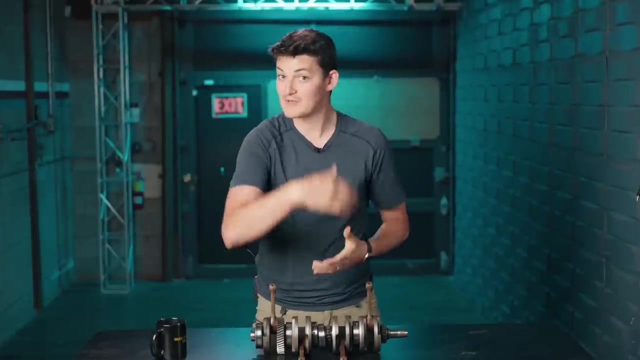 and enough airflow to avoid stalling under the fully grown van. The new school might start on massive four-strokes that can lug around at 2,000 RPM all day, but that does not mean it's a good idea. How many revolutions per minute does your engine prefer? How many RPMs should you prefer? Why do? 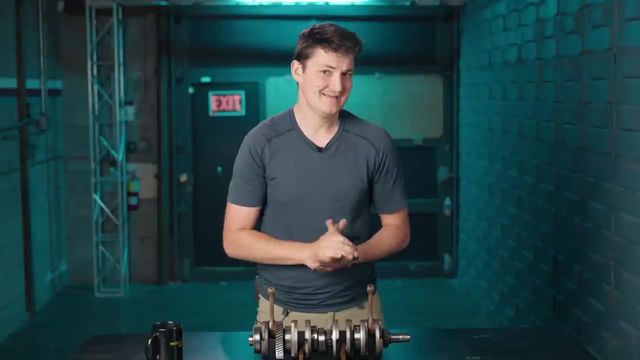 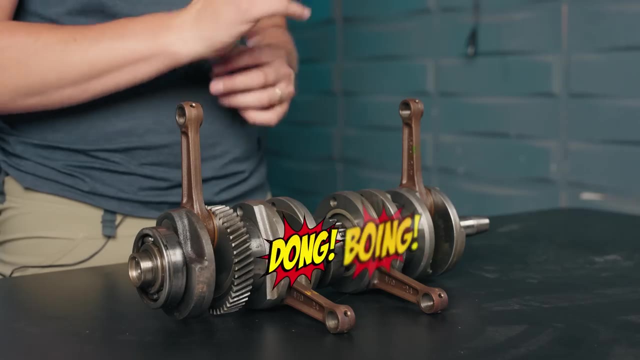 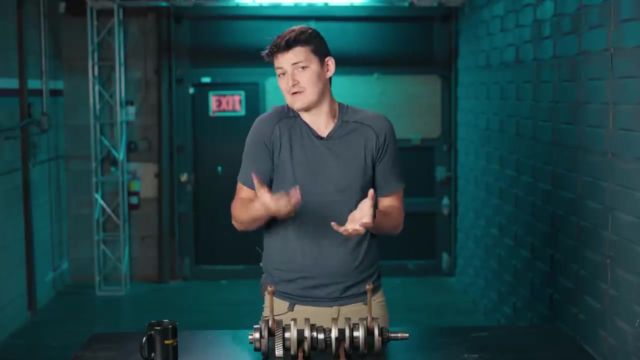 bicycles exist. These are not subjective questions and today we find answers In engineering terms. a four-cylinder goes bang, boing, dong, ding, while the crankshaft goes round and round the mulberry bush. Now, I'm no engineer. I studied physics like a grown-up, but even I know that 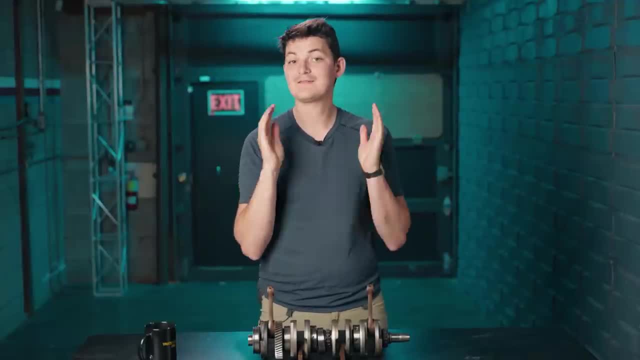 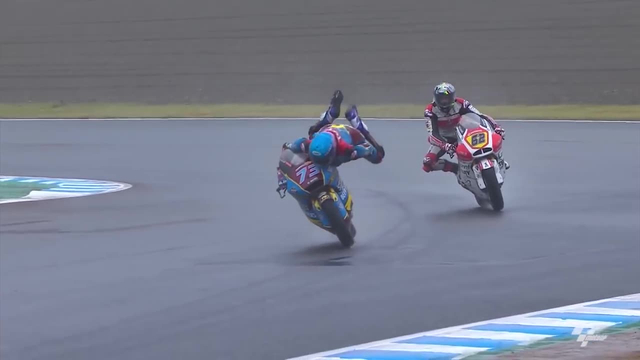 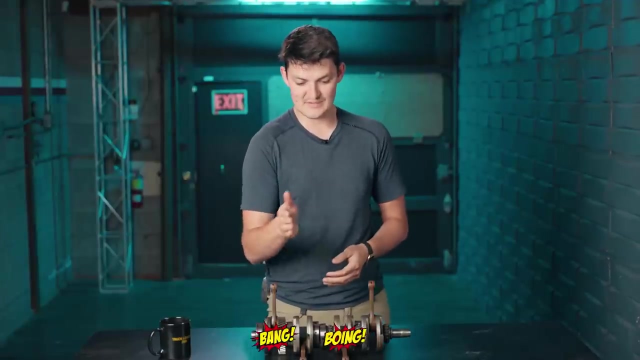 when the crankshaft spins faster than required, you get a spontaneous system rebalance. That's why we have traction control. The computer decides to go: bang boing, dong nothing, nothing, nothing, dong ding, nothing, nothing. TC cuts power, pulses. 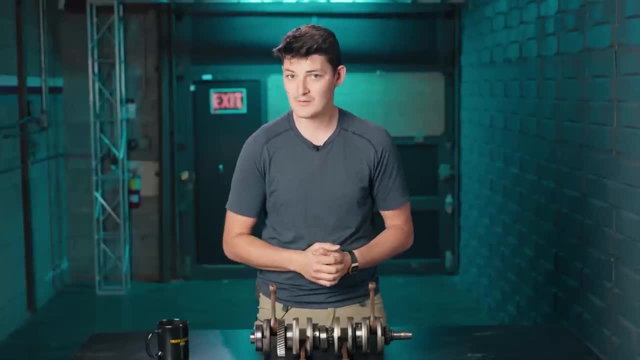 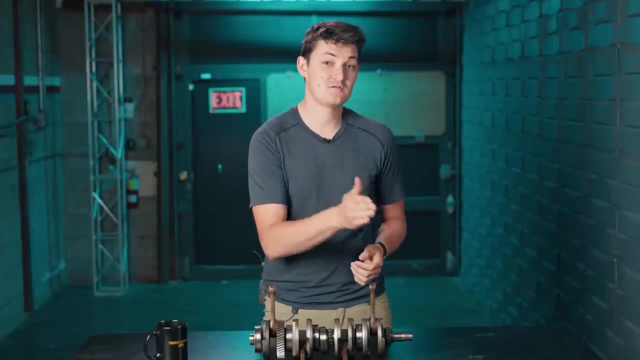 until our crankshaft is back in time. with our rate of travel In six gear at 2,000 RPM, you're giving the computer fewer opportunities to correct your mistakes. In third gear, at 8,000 RPM, suddenly our traction control works four times faster. 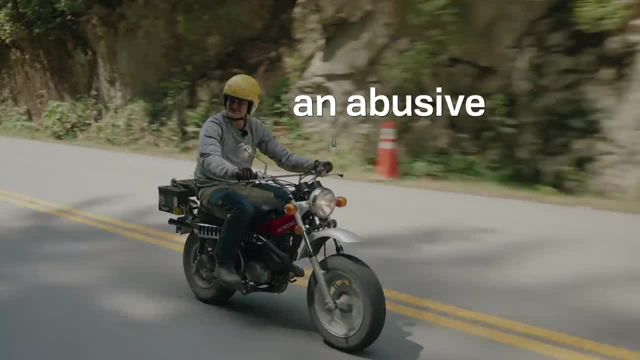 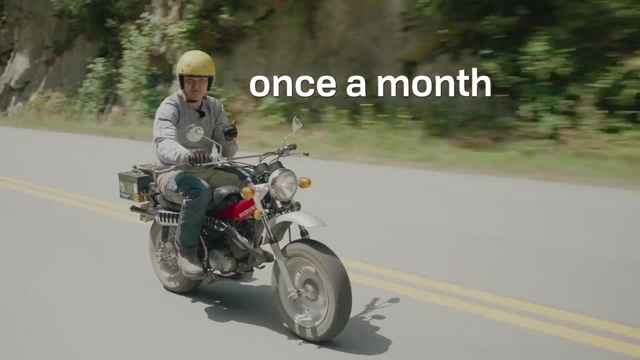 If you still think 7,000 RPM constitutes an abusive relationship, consider the. Consider the Italian Tuna. I bought this bike from an elderly gentleman who used it once a month to collect the last crumbs of our Canada pension plan. I swear to David Suzuki. 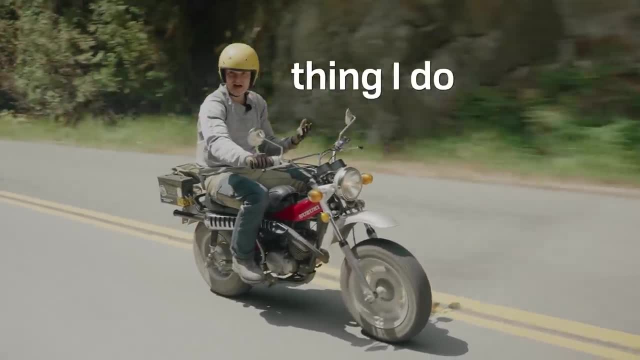 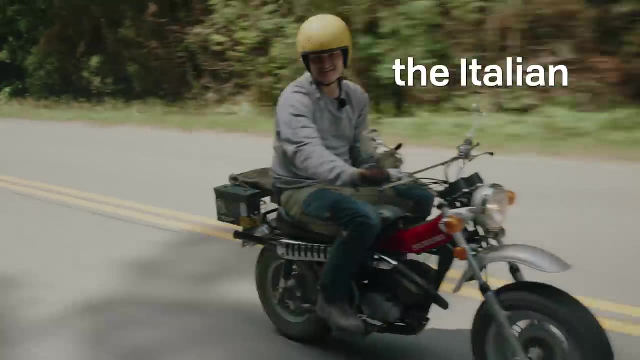 he made free horsepower when I bought it. The first thing I do is that I did like the valentino a rossi, because I love a boogie, And they call that the Italian Tuna. Now, I reckon this engine contains as many horses. 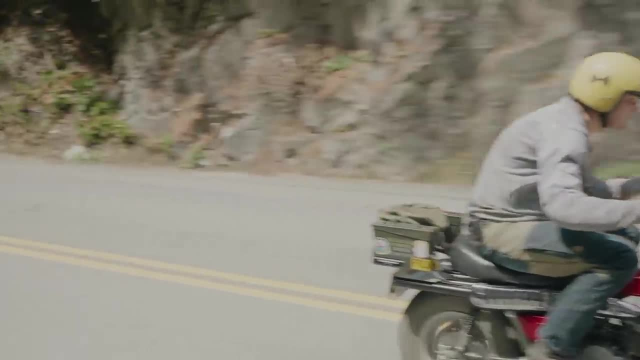 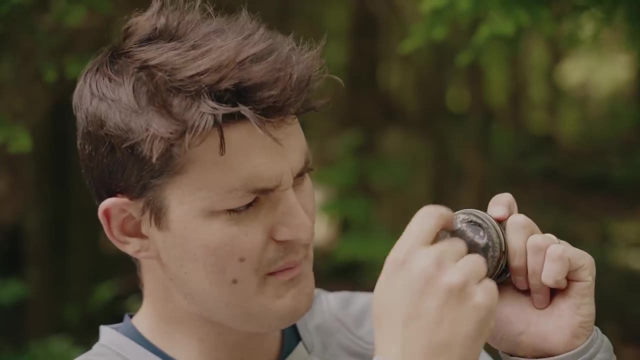 as a six pack of Ikea meat balls, But I'm not sure if it's the right word for it: Bold claim. so let's explain. At 200 degrees Celsius, carbon starts to form deposits in your engine And this buildup eats away at your compression ratio. 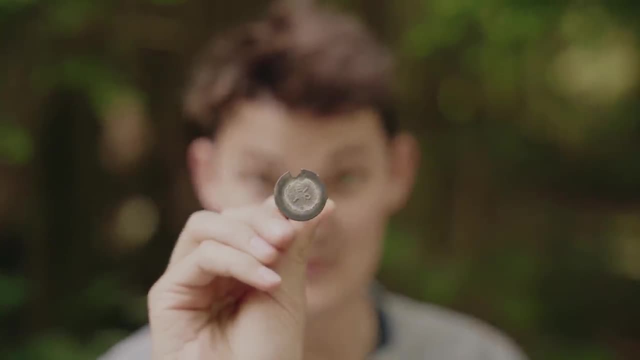 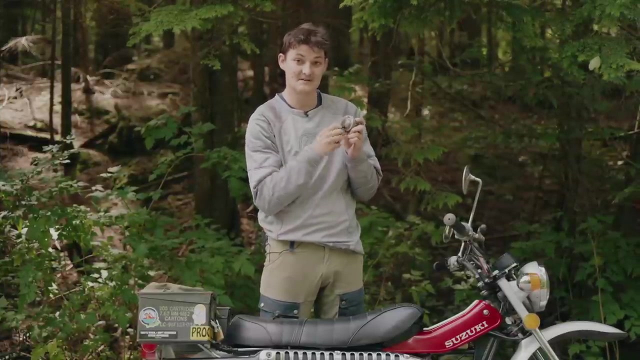 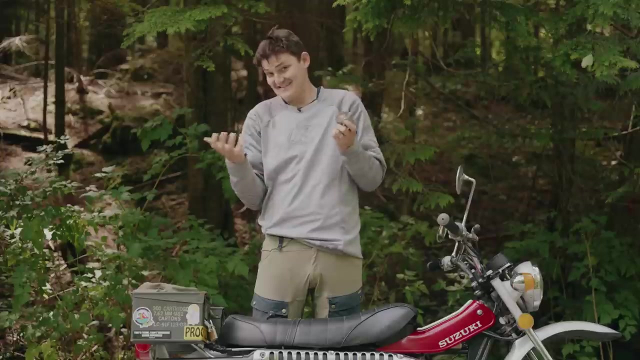 and, if left to grow, can prove fatal. But at 325 degrees Celsius that carbon starts to break apart again And, subjected to fast enough airflow, will blow right out of your exhaust. So riding at high RPM does theoretically clean your engine. 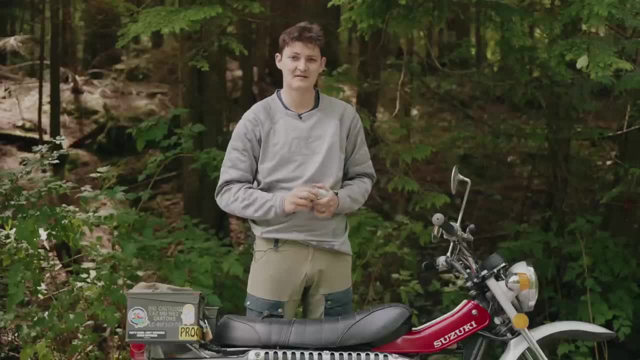 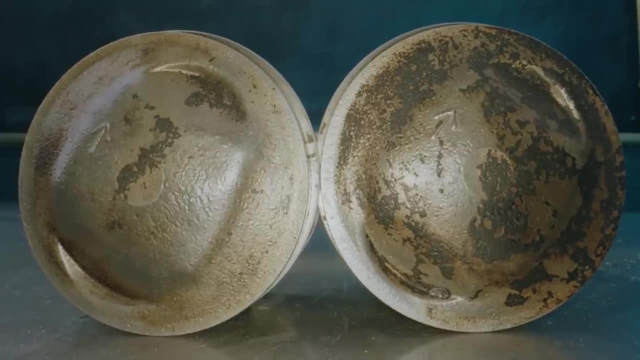 Empirically I've had success with many barn, find Italian tune ups. but anecdotal evidence is only evidence of an anecdote. So look, one piston ridden hard, one ridden soft. If you're still uncomfortable hearing your bike sing, consider metal stress. 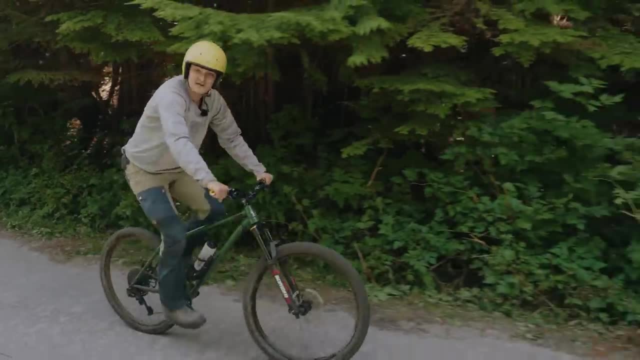 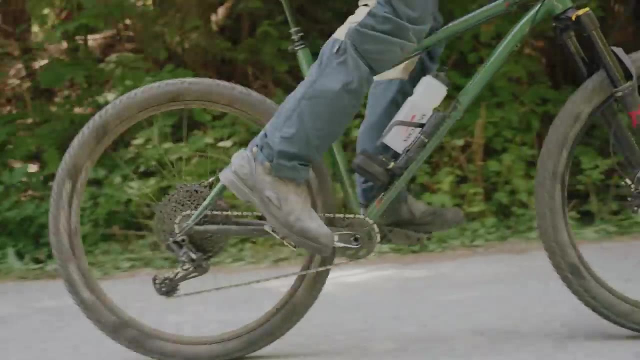 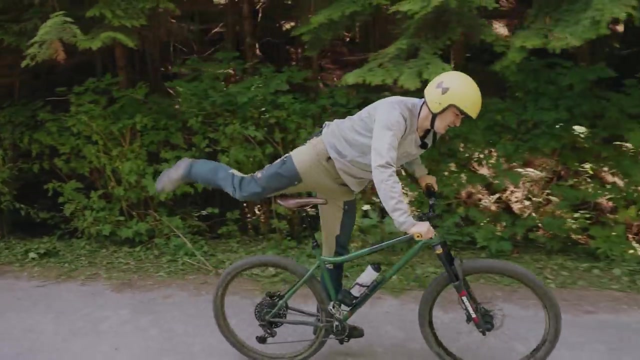 And at high RPM my pedals- I mean pistons- don't have to push very hard on my cranks, I mean rods. But at low RPM, the same speed. woo, That's a lot of force. Woo, I guess it's like a pretend motorcycle. Gross. Think of it this way: your combustion always has the same energy. High RPM gives that pressure somewhere to go, low RPM does not. It's a catch-22.. High rev sends the pistons on more reps than necessary. you're kind of wearing your engine further than. 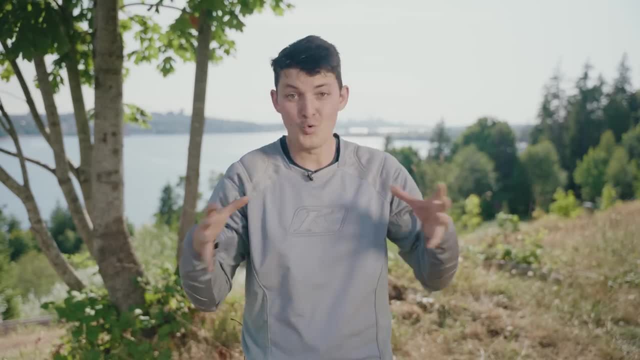 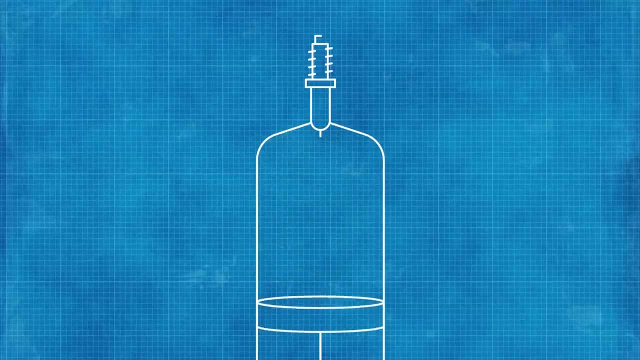 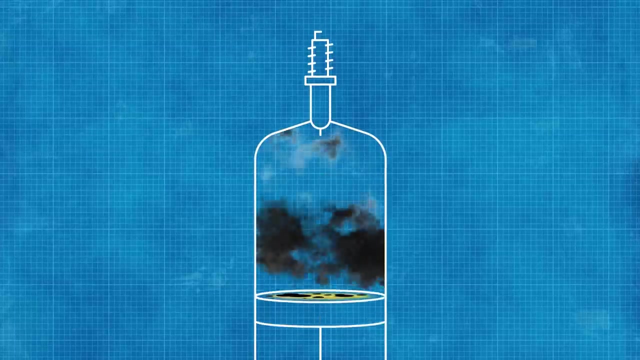 its odometer reading. But low rev exerts more cylinder pressure. Between the two evils, that's the greater danger. See, add it all up. Low RPM leaves carbon deposits. Low RPM requires the pistons to push harder, creating local hotspots, And the slow rotations mean more time. 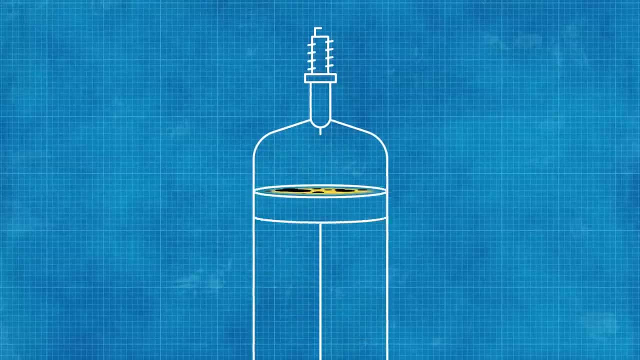 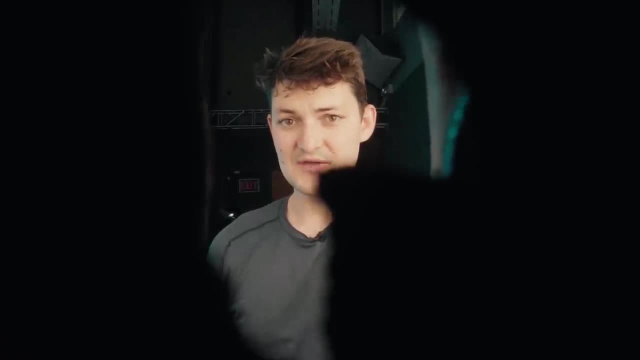 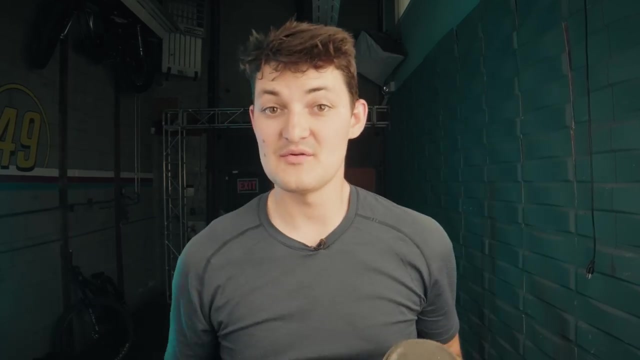 spent in the dangerous pre-ignition phase One flare-up while the piston is still rising, kaboom. They call this low-speed pre-ignition or detonation. Never lug your engine. Now go forth and rev the tits off your motorcycle. The metal is healthier at high RPM. The traction 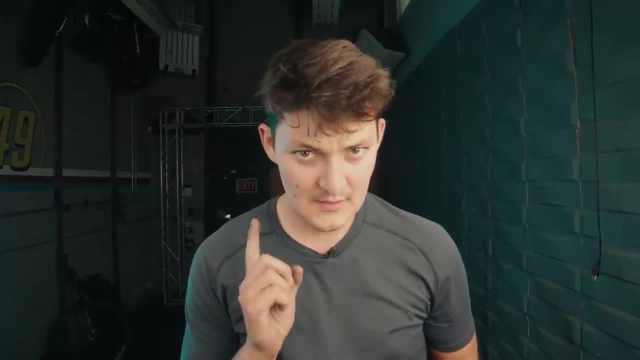 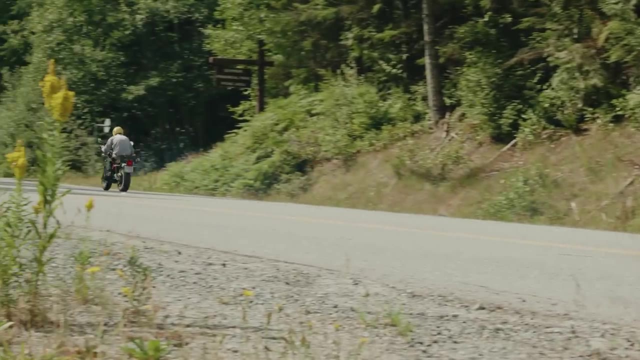 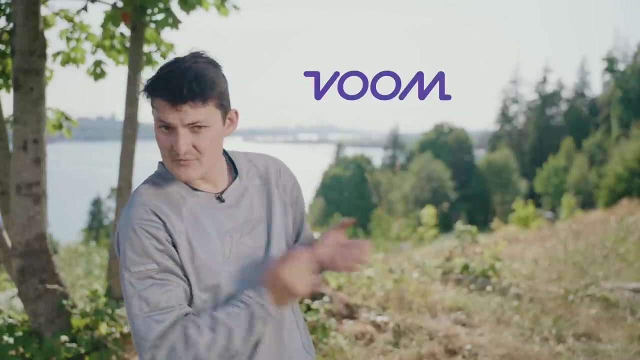 control is faster at high RPM. You paid for the whole tachometer, so use the whole tachometer. Thank you very much for watching and thanks to VOOM for sponsoring our video. If you haven't made a quote already, please do me a favor and make one. It's the industry.